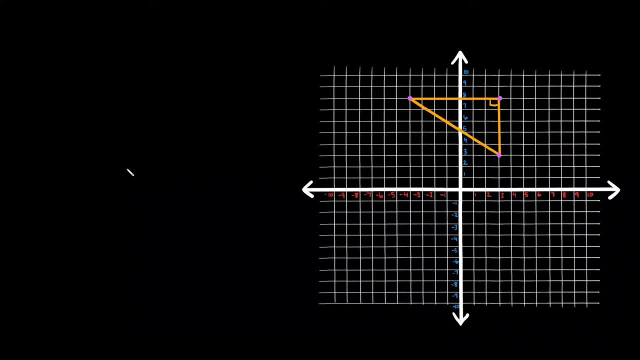 What's up, you freaking geniuses? So in this video, I'm going to teach you how to find the perimeter and area of shapes and polygons in the coordinate plane. All right, so, first of all, we have a triangle right here. right? so the area of a triangle, of any triangle, is equal to one half the base times, the. 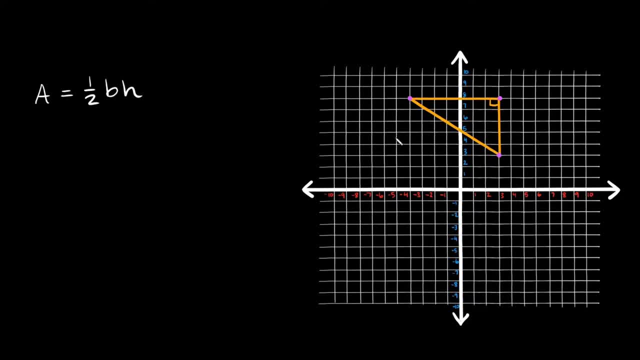 height. Okay, now, when your shapes are lined up with the grid like this, it's a little bit easier to figure it out. okay, because, as you can see, the base right here would just be this horizontal side, right. so the base. how long is the base? well, it's one, two, three, four, five, six, seven, so it's seven. 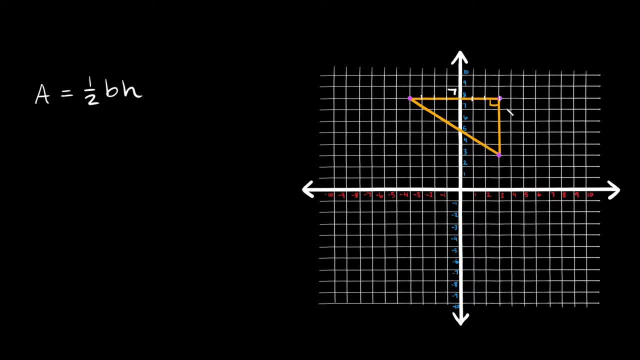 spaces long, or seven units long, and then the height would be right here. right, so the height would be one, two, three, four, five. okay, so it's five, right there, okay. so if we wanted to find the area, the area would be equal to one half the base, which is seven times the height, which is five. 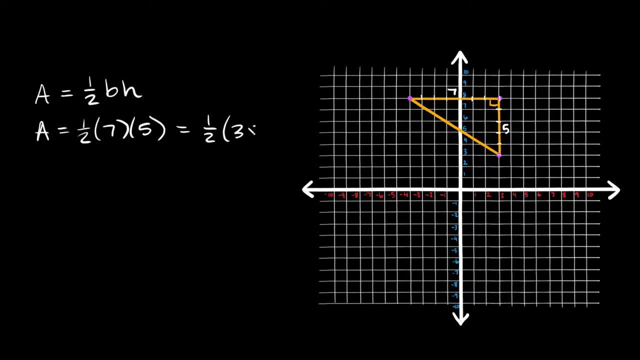 okay. so it'd be equal to one half times thirty five, which is equal to seventeen point five. okay, and whatever your units you're using, just put those there and then they would be squared, right. so we'll just say seventeen point five, units squared, okay. now, in order to find the perimeter, we have to add up all the sides together, right? 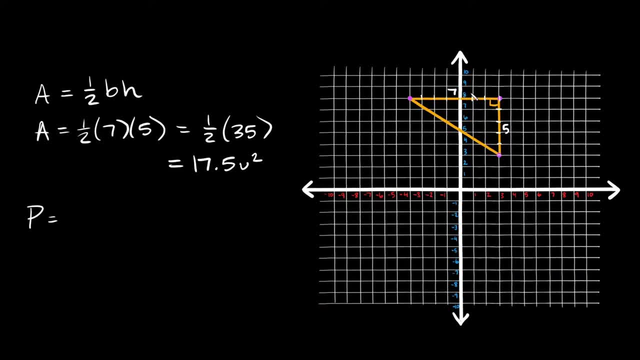 so we already have these two and, if you notice, we can actually use the pythagorean theorem to figure out this missing side. right here, the the hypotenuse, right here, right this long side. so the formula for that would be: a squared plus b squared is equal to c squared. okay, where a and b right here are your two shorter. 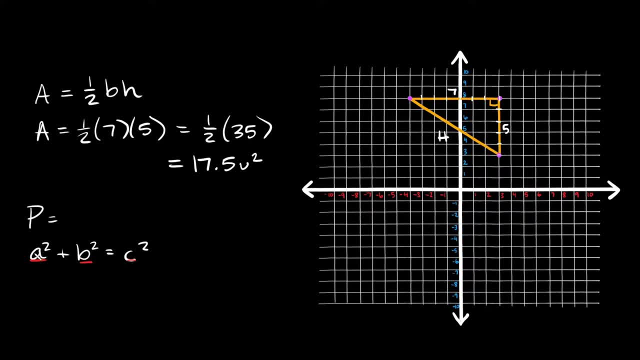 sides, and then c is your hypotenuse, okay, so first of all, uh, we can plug in. let's see, we have a seven and a five. those are our shorter sides, right? so we can plug in a seven here and a five here, okay? so then we'll have seven squared plus five squared is equal to c squared. okay, now, seven squared is equal. 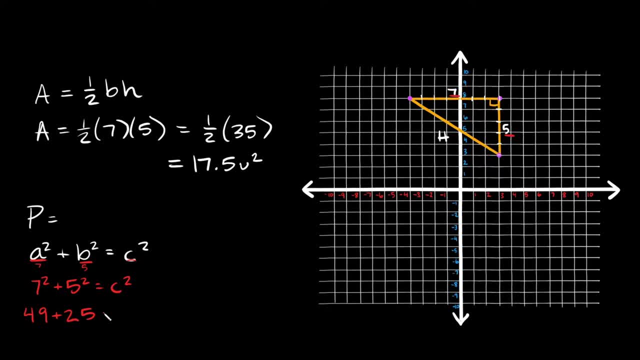 to forty nine. five squared is twenty five, and that's equal to c squared. okay now, forty nine plus twenty five is equal to. well. forty nine plus twenty is sixty nine. nice plus five is seventy four, okay, so here we have. seventy four is equal to c squared. okay, now to get rid of this exponent. right here, the two. right, we have to take the. 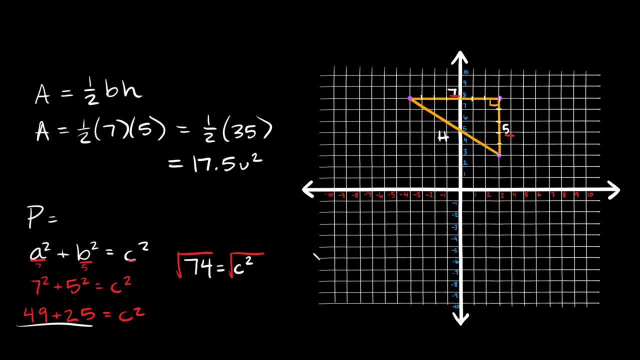 square root of that, and what we do to one side, we do to the other right. so then here these cancel out. so then on this side, we're just left with: c is equal to the square root of seventy four, which is approximately- let me change my symbol too- then approximately 8.6, all right, so. 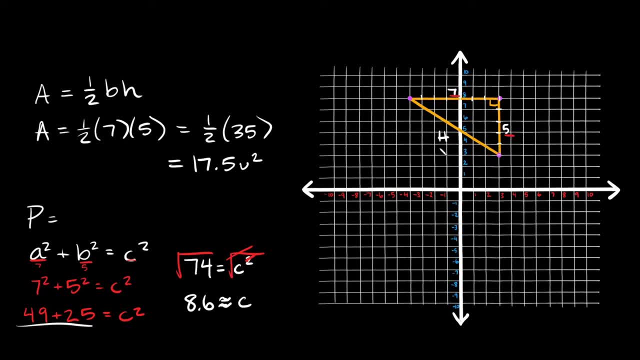 this side. right here is the hypotenuse. we're going to say it's about 8.6. okay, now, if we want to find the perimeter, now we can add up all the sides together. right, so we're going to have 7 plus 5. 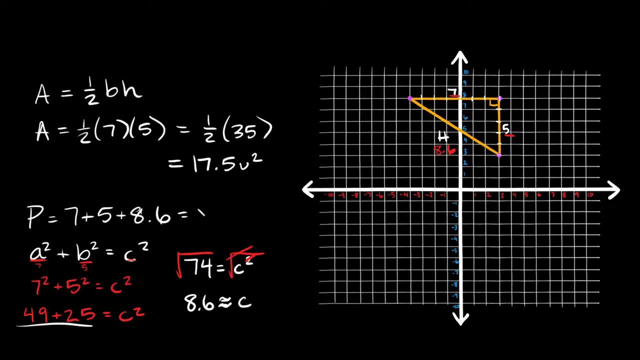 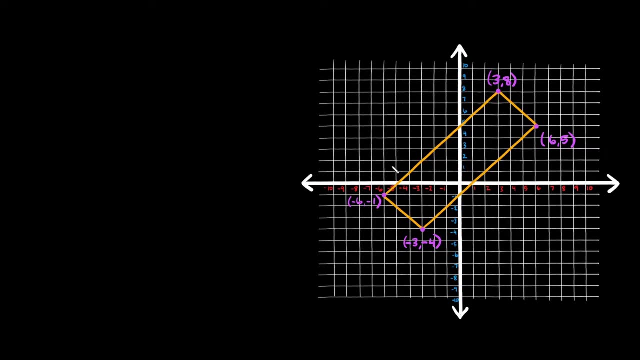 plus 8.6 and that's equal to 20.6. and if we have units here, you know, you just write your units right right: inches or feet, miles, whatever. okay, so here's the perimeter, all right. so here's our next example. so we have a rectangle, right. so the area of a rectangle is the length times the width right. 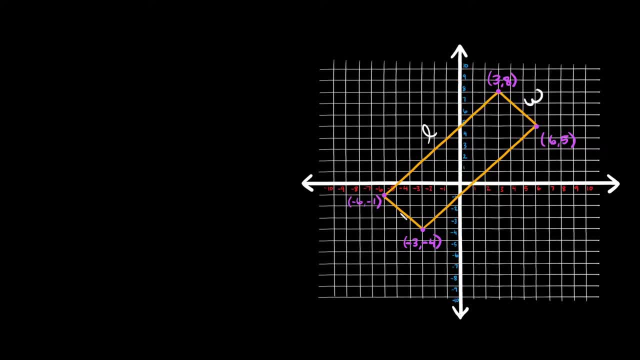 so in order to find the area here, since it's at an angle right, it's not lined up with the grid- we can't just count spaces like we did last time, so in this case we're going to have to use the distance formula. now, if you don't remember what that is, i'll write it right here. so it's x of 2 minus x of. 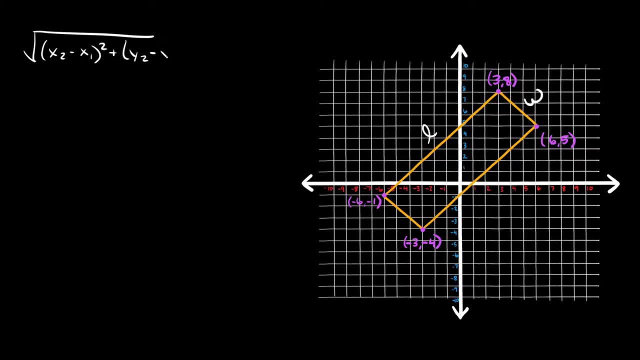 1 squared, plus y of 2, minus y of 1 squared. okay, so this whole thing is under a square root. okay now, if you're not familiar with this, i'll link a video to that in the card above. but this is the formula you have to use in order to find the distance between two points. okay, so if we want to find 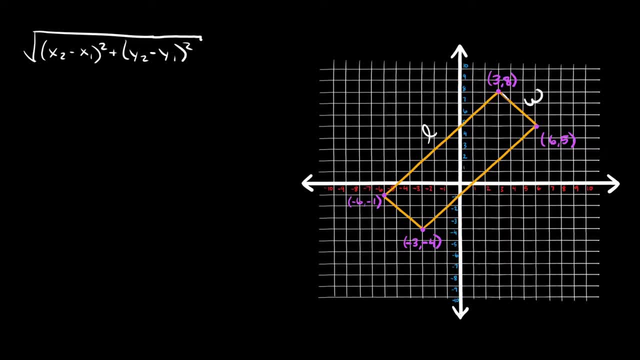 this side, right here, this length. we have to find the distance between these two points right here, right three comma eight, and negative six comma negative one. okay, so So if we're going to use the distance formula, we have to label our points here that we're. 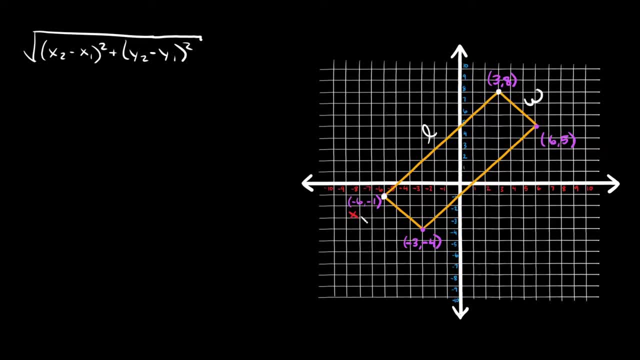 going to use. Okay, so this one, let's label this one as x of 1,, y of 1, and this one we'll label as x of 2,, y of 2,. okay, So now that we labeled our two points right here, now we can find the distance between. 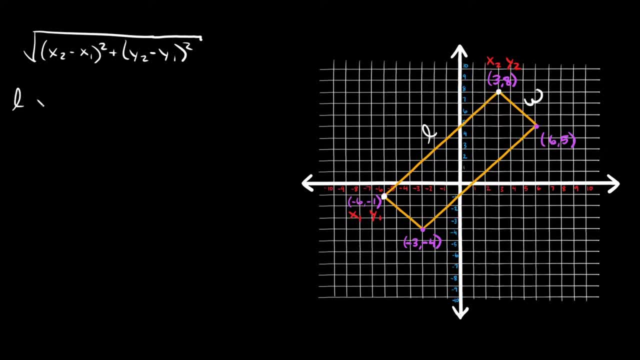 them, okay, By plugging it in right here. So we're going to have: the length is equal to the square root of all this junk, right here, right? So x of 2 minus x of 1.. So we're going to have x of 2, which is 3,, minus x of 1, which is negative 6.. 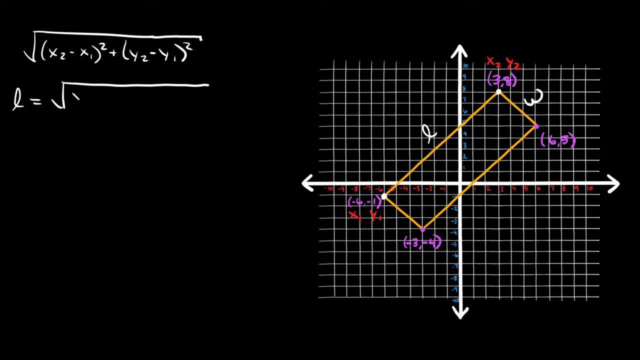 So 3 minus negative 6.. Okay, so in parentheses we're going to have 3 minus negative 6, and that's squared. And then we're going to add that to our other set of parentheses right here, y of 2 minus. 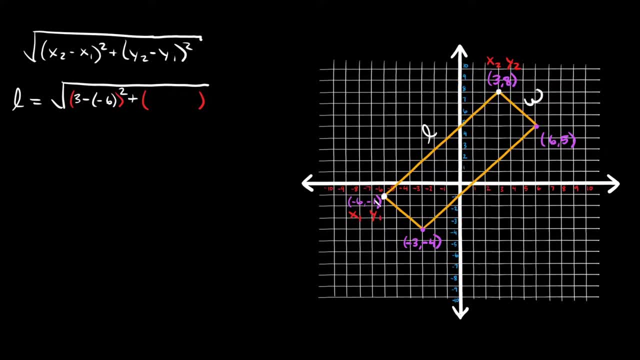 y of 1.. So y of 2 is 8, y of 1 is negative 1.. So we're going to have 8 minus negative 1, and this is also squared, okay. So then this is going to be equal to the square root of now 3 minus negative 6, that's the. 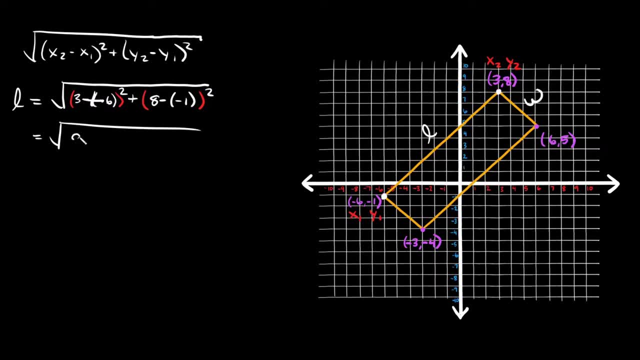 same thing as 3 plus 6, right. So 3 plus 6 is equal to 9,. okay, So we have 9 squared, and then we're going to add that to here. So 8 minus negative 1, so this is the same thing again as 8 plus 1.. 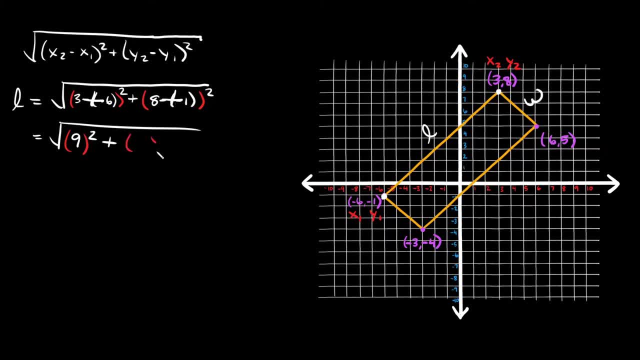 So 8 plus 1 is equal to 9 squared also. right, So 9 squared also okay. So then here we're going to have the square root of: well, 9 squared is equal to 81, right, So we have 81 plus 81, which is equal to the square root of 162, which, if you plug into, 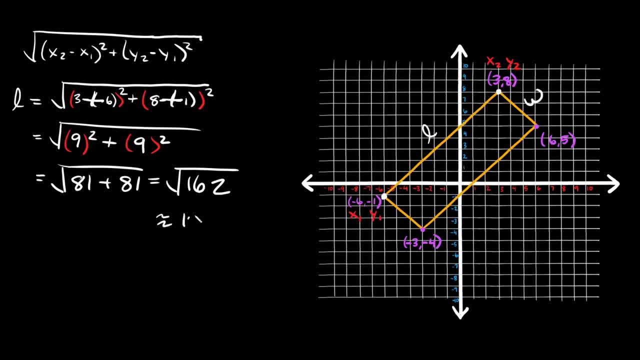 your calculator, you're going to get approximately 12.7, okay. So the length right, the length right here, the distance right here is equal to approximately 12.7, okay, Now we just have to find the width right. 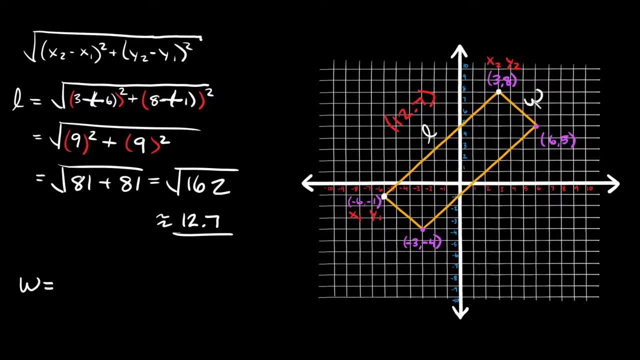 So, again, we're going to use the distance formula to find the width, okay, And to find this side, We're going to use these two points right here: right, 3 comma negative 8, and 6 comma negative 5,, okay. 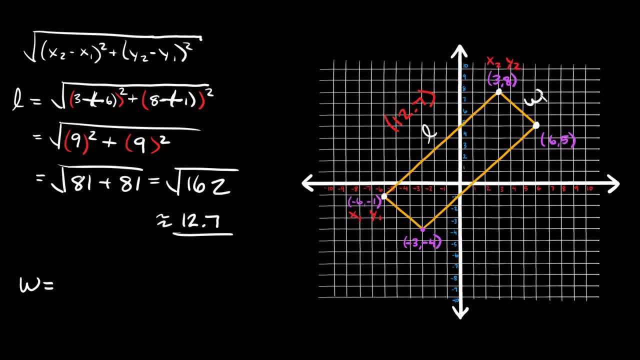 So this one, since it's already labeled, I'll just leave it as x of 2, y of 2, and then this one will be x of 1, y of 1, okay. So these are the two points we're using this time, okay. 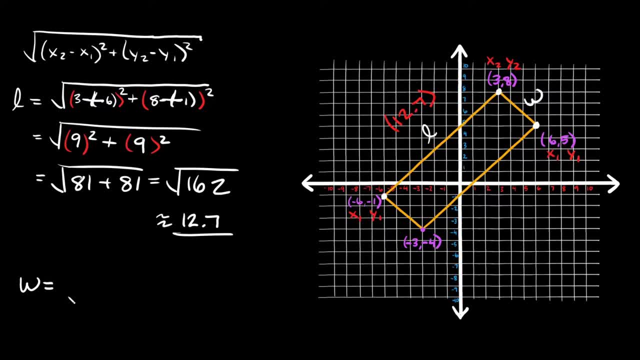 So now that these are labeled, now we can plug them into our formula right here. okay, So we're going to have the square root of: remember, it's x of 2 minus x of 1, right? So x of 2 is 3, x of 1 is 6.. 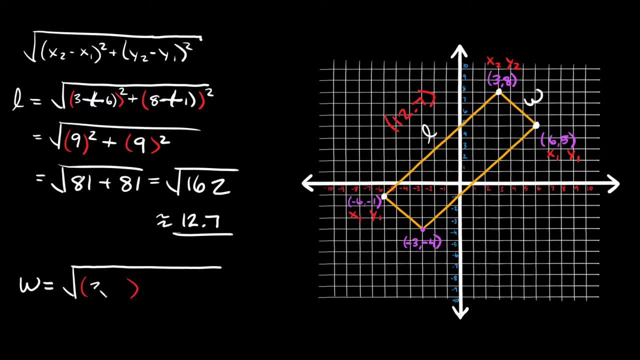 We're going to have 3 minus 6 in our first set of parentheses right here, right, 3 minus 6, and that's squared. and then we're going to add that to this set of parentheses right here: y of 2 minus y of 1.. 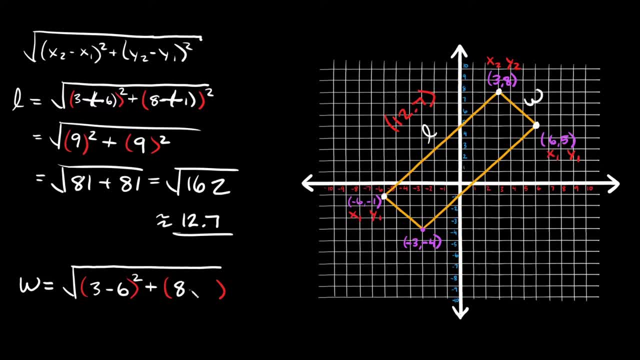 So 8 minus 5,, okay, 8 minus 5, and this is squared also, okay. So then the width is equal to the square root of 3 minus 6,, that's equal to negative 3, and this is squared plus 8 minus 5,, which is equal to 3, and that's squared also. 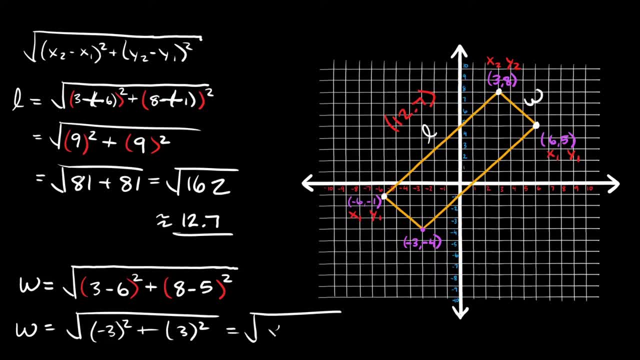 So then we have the square root of negative: 3 squared is equal to 9, and 3 squared is equal to 9,. okay, So here we have the square root of 18, which, if you plug that into your calculator, you're. 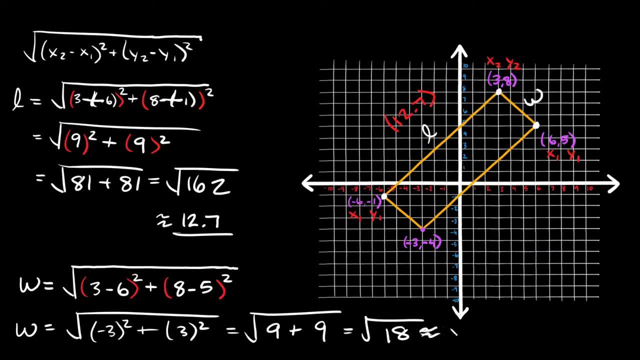 going to get about right- approximately 4.2, okay, So then the width over here is approximately 4.2,. all right, and let's get rid of all this crap in 3,, 2, 1, boom, all right, cool. 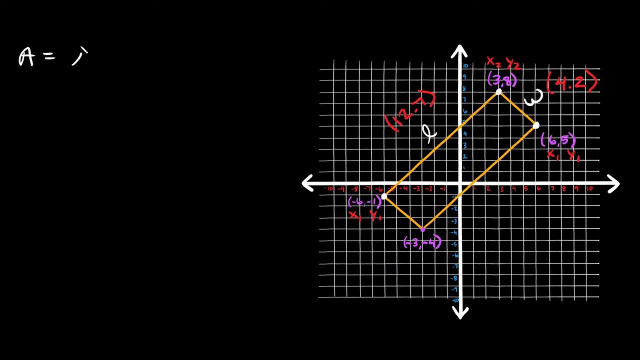 Now in order to find the area, Remember, the area is just the length times the width, right? So here we have 12.7 times 4.2.. So 12.7 times 4.2, and that's going to be approximately, again right, because we're. 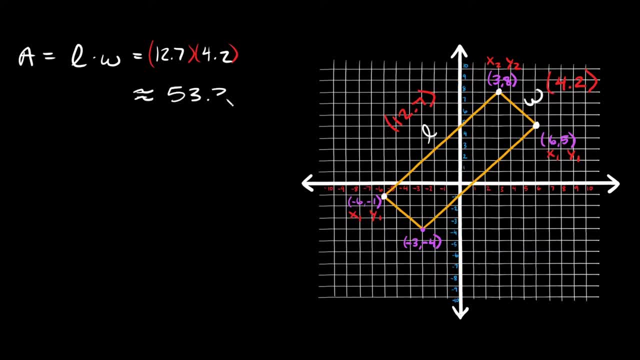 just rounding everything: 53.3, and those are units squared right. Don't forget those. all right, So that's the area, right here. Now to find the perimeter, remember, we just have to add up all of that, All the sides, right. 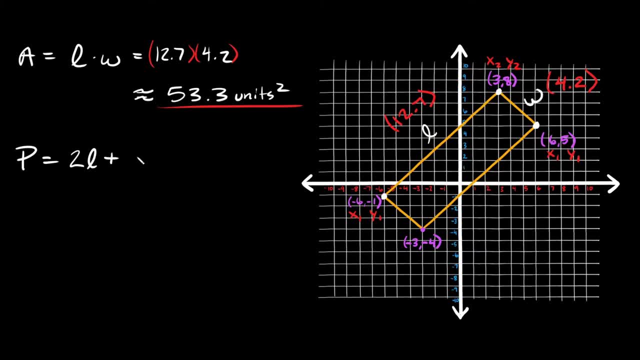 And another way we could write that is 2 times the length plus 2 times the width, okay, So then the perimeter is going to be equal to 2 times the length, which is again approximately 12.7, right, plus 2 times the width, which is about 4.2, okay. 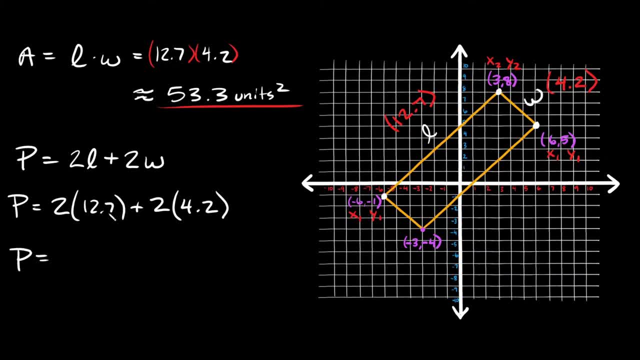 And then the perimeter, so 2 times 12.7, that's equal to 25.4, plus 2 times 4.2, so then this is equal to 8.4, right, And if you add these up you're going to get a nice grand total of 33.8 units in length. 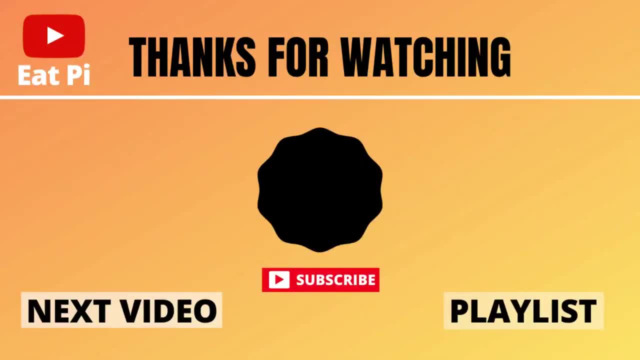 all right. So then that's your perimeter. So if you found the video helpful, definitely leave a thumbs up down below, and if you have any other questions or want to see any other examples, just let me know in the comment section below.